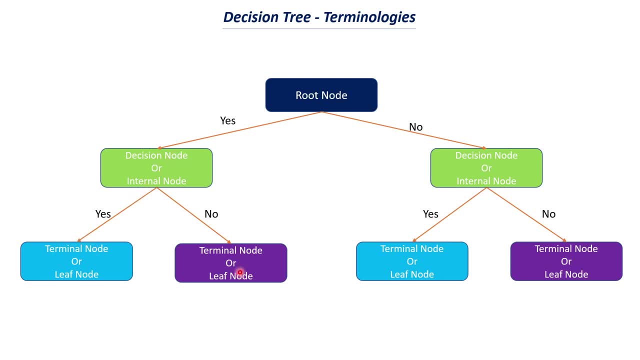 data set. So this will go on until it reaches a terminal node or leaf node. So in a decision tree you have root nodes, you have multiple terminal nodes and leaf nodes, and in the decision tree you will have any number of decision nodes or internal nodes. So this is how a 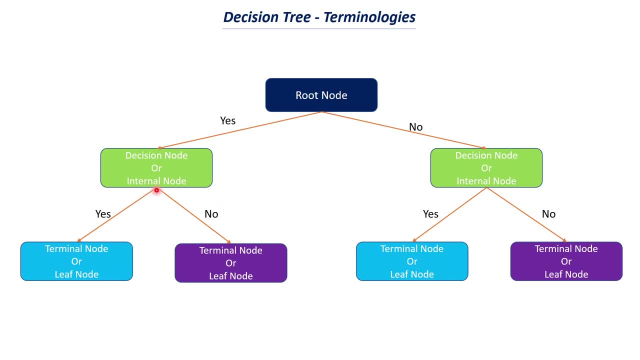 decision tree looks like when you just visualize it. Now we need to understand which feature we have to choose for root node and which feature we have to choose for internal node and terminal node, and so on. So this is where the measures such as entropy information. 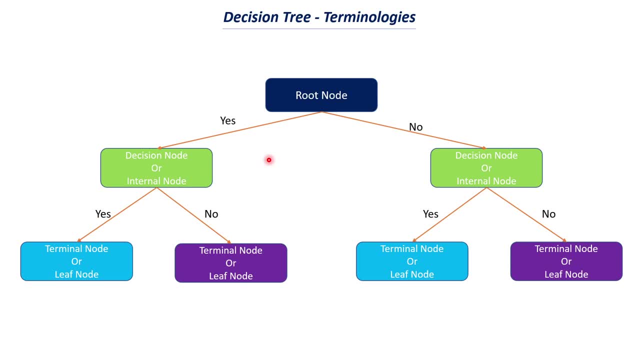 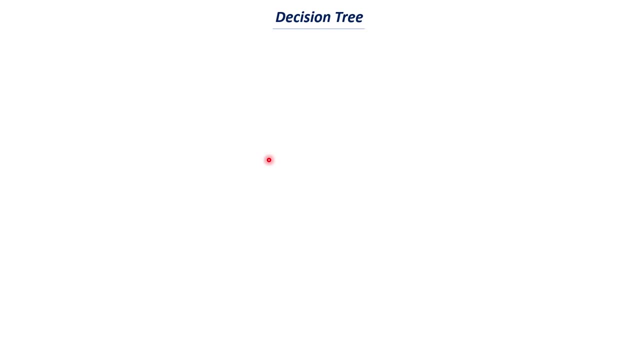 gain and Gini impurity will be helpful for us. So they are like the measures, which helps us to decide which features we are going to choose when. So let us try to understand this with an example. Let us say that we have a problem. 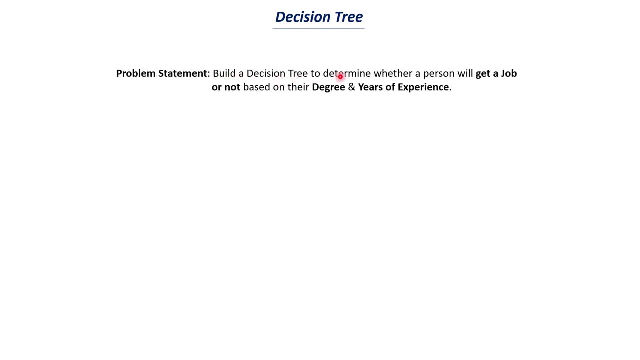 statement and the problem statement is: we have to build a decision tree to determine whether a person will get a job or not based on their degree and years of experience. Here the degree and years of experience are features, So these two are our features and you can. 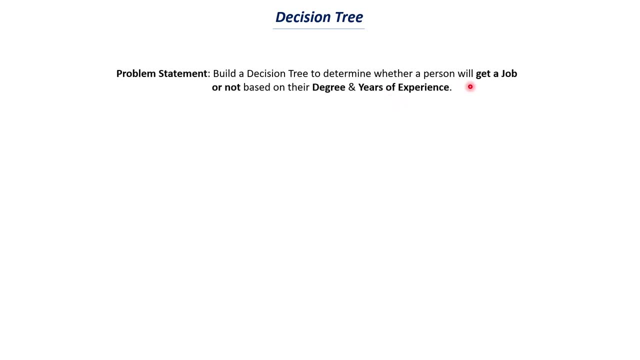 also call these as independent variables, And we are trying to predict whether a person is going to get a job or not, whether they are going to be placed or not. So this is our target variable, or you can call this as the dependent feature, because whether a person 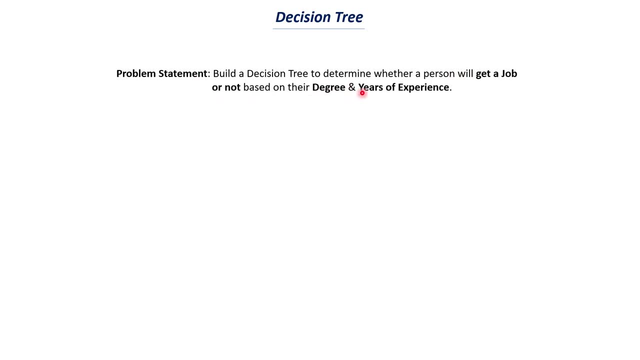 is going to get a job or not will depend on what you are doing during the day or, if you, What is the degree and years of experience in this particular case? Okay, So let's say that this is the small data set that we have for this case. 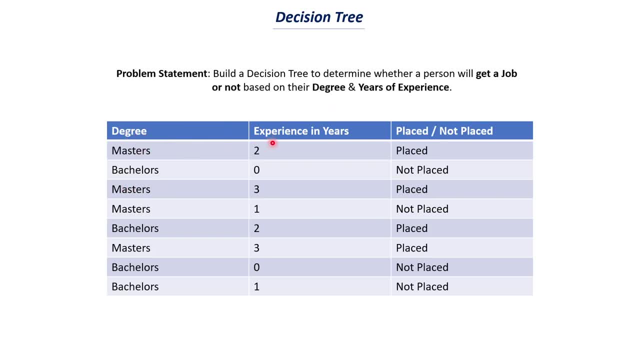 So we have the degree of several people here, their experience in years and whether they are placed or not, Okay, So whether they did masters in engineering or bachelor's in engineering and so on. So totally we have about 8 data points here and this tells us what is their work experience. 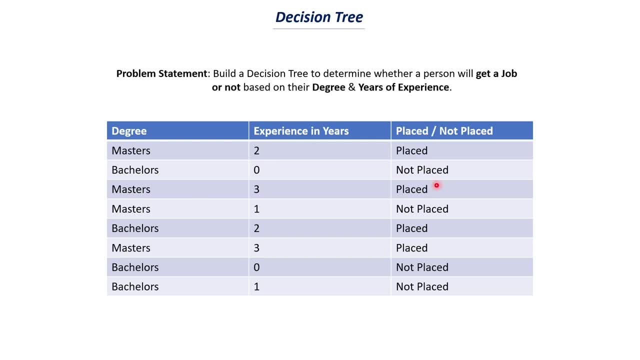 in years and, finally, whether they are placed or not. Okay, So this is the data set that we have, and now we need to build a decision tree that can use this features, degree and experience- in order to find whether a person is placed or not. 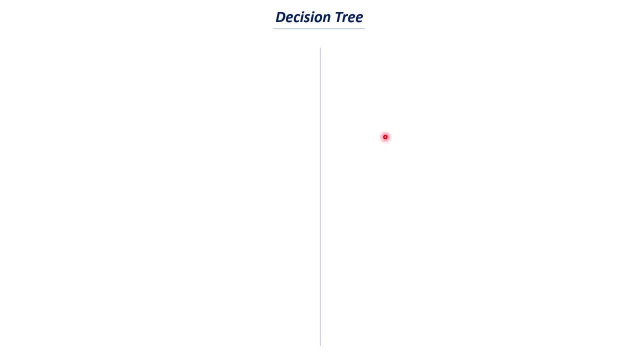 So let's see how we can build this decision tree. So in this case, we will be building two decision trees and comparing their prediction. So which decision tree we have to choose as our final model, and so on. Okay, So let's say that this is the first decision tree we are taking. 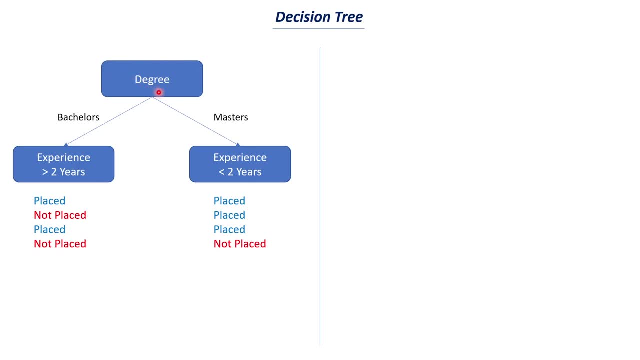 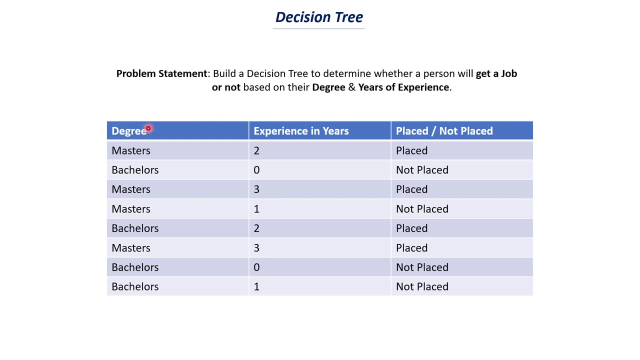 So this is our root node, right? So in this case I am choosing my feature, degree, as the root node. So, as you can see, here we have two features, which are degree and years experience in years. So in the first decision tree We will choose degree as our root node and in the second decision tree we will choose 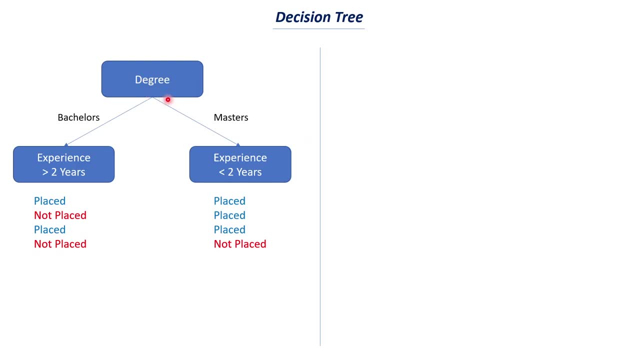 experience in years as our root node. So, as you can see, we have a degree as our root node and the two possibilities in this case are bachelor's and master's. So we call this as splitting. Okay, So we are splitting this particular attribute into two splits. 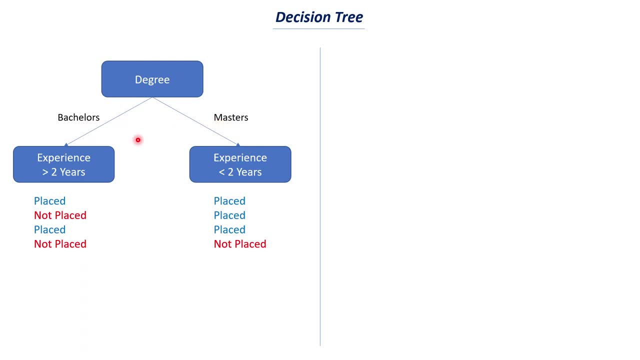 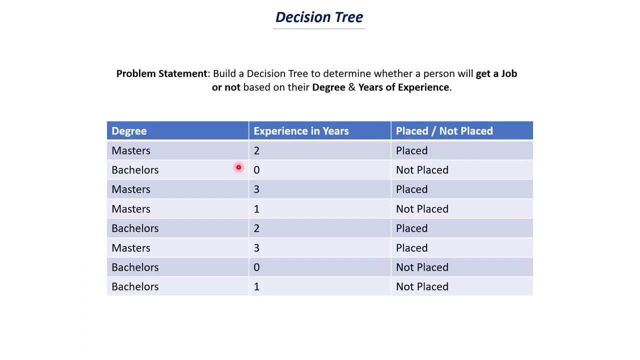 One is whether a person has completed bachelor's or not, or whether they are completed master's, and then we are checking whether their experience is, you know, greater than two years or less than two years. So we cannot use this continuous values directly, So we need to, you know, categorize them in some way. 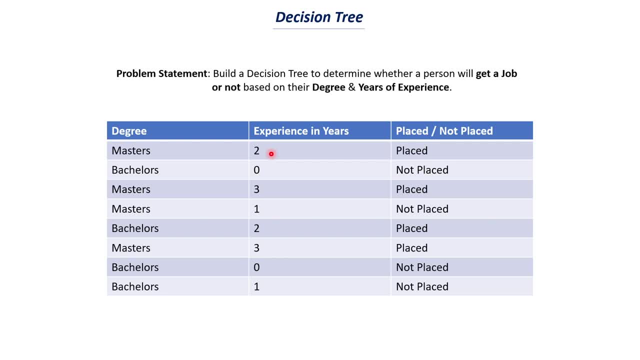 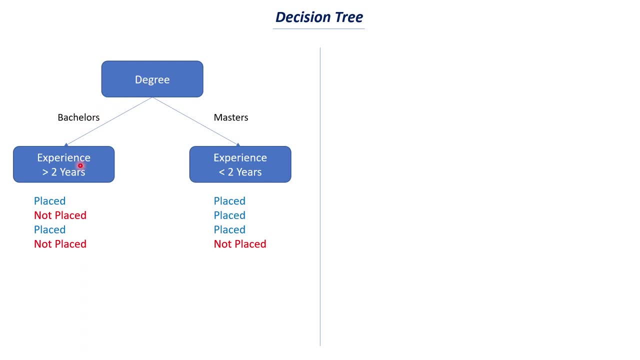 So we are going to categorize whether the experience is greater than two years or, you know, less than two years. So that is the decision boundary we are, you know, building. So let's say that if a person has completed bachelor's and they have greater than two, 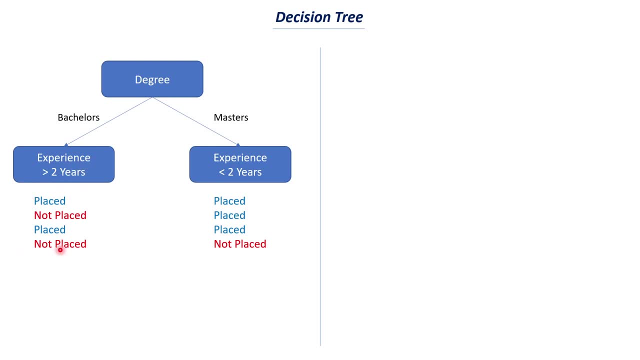 years of experience. This is the case. So, out of these four people, So like these four people have completed bachelor's of engineering and they have, you know, greater than two years of experience. So we can think about like that: and out of these two people are placed, and two people 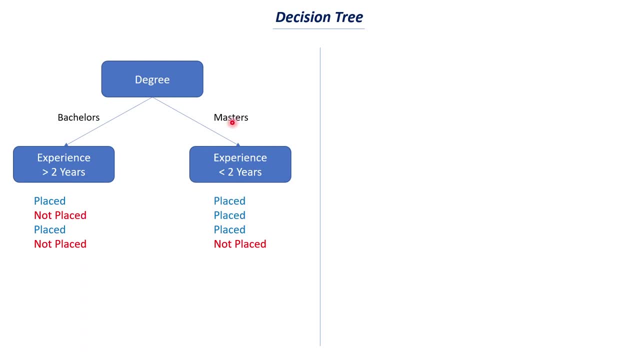 are not placed. So, if you consider this, So there are four people who have completed master's And Of course You know they are like less than two years of experience. out of this particular class, three people are placed and one person is not placed. 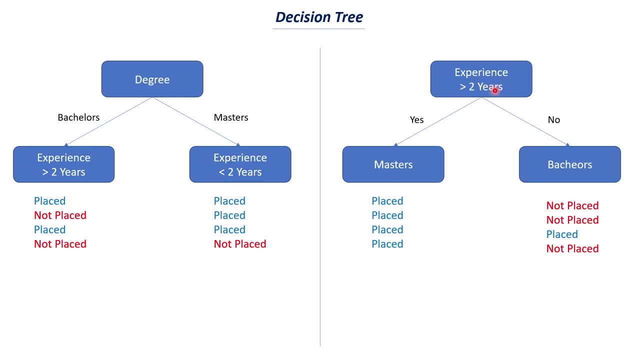 So, if you consider the second decision tree that we are building, in this case we can choose experience in years as the root node. so, instead of degree, we can use this experience in, you know, greater than two years as a root node, and we are checking whether this condition 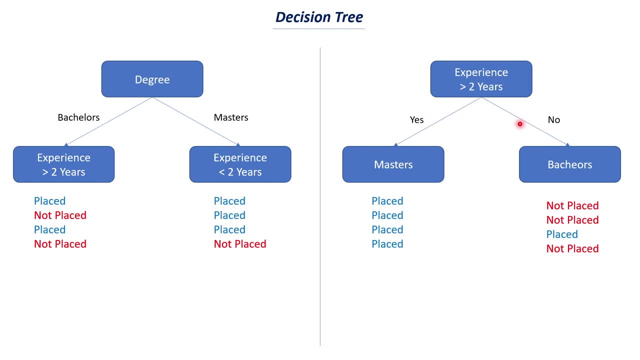 is yes or no. So no means they are. the experience is less than two years. Yes means it may be like three or four or whatever. it is OK. So if they are masters, we can see that four people are placed And the bachelors. there are only three people. not only one person is placed and three people. 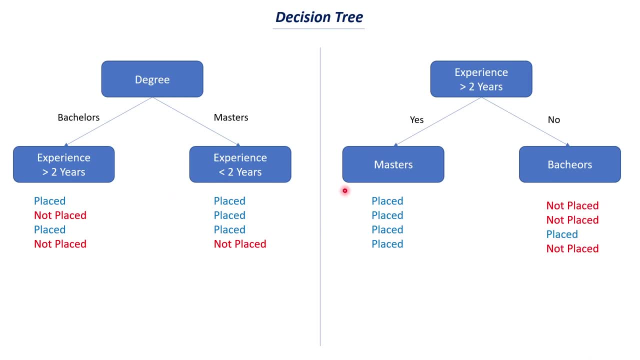 are not placed. So this is the decision tree that we are getting, OK. So, to be honest, if you just compare it to the data set that we have, this may not add up, but that is not the point, OK. So I just want to build this for explanation purpose. 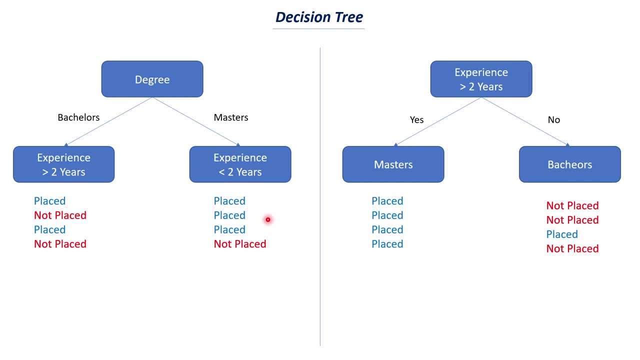 So this may not add up. so you don't need to go through the data set exactly and see whether it is correct or not. OK, Because, like, if we build an actual decision tree, we will include another yes or no branch and then we will see whether the person is placed or not. 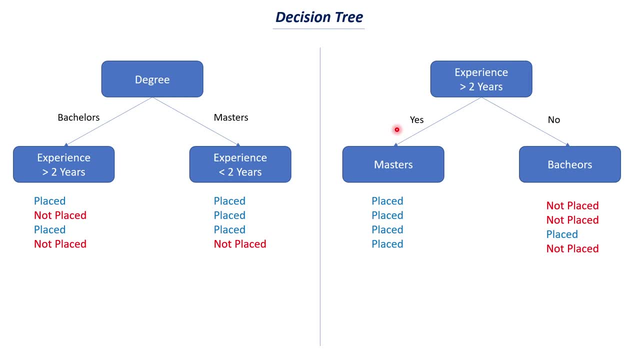 So if you do that, The decision trees will be kind of the same thing. So for explanation purpose, let's say that this is the final output we are getting, OK, So you don't need to look at the data set. So if a person has completed bachelors and they have a greater than two years of experience, 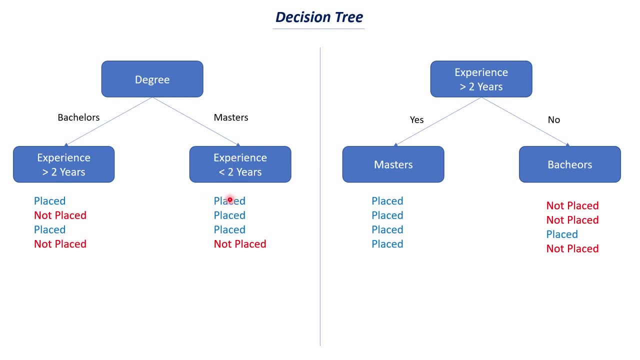 this is the result. So two is placed and the two is not placed, and experience is less than two years. Three people are placed and one person is not placed. So when you have this decision tree, how you can make a new prediction is that you can. 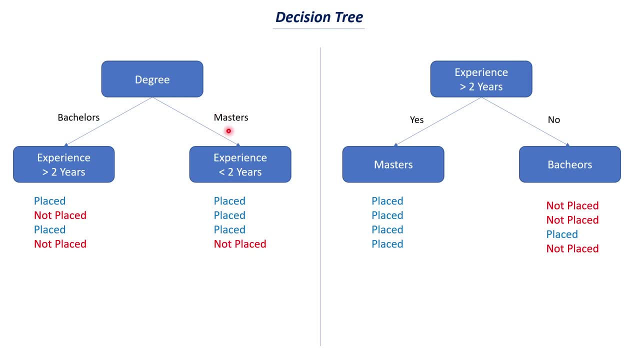 ask whether that person is, you know, completed masters or not. So if that person has completed masters and if they have, you know, experience less than two years or even greater than two years, there is a high probability that they are going to get placed. So if they are completed bachelors, the probability that they are going to get places, kind of. 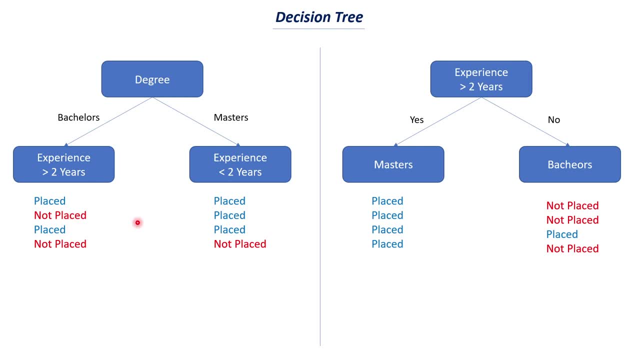 50 percent chance and something like that. So this is how we can use this decision tree in order to make predictions. Now we have used the same data set, we have used the same features, but we have interchanged the position of these features. So, in this case, degree is my root feature, or in other words, is my root node, whereas 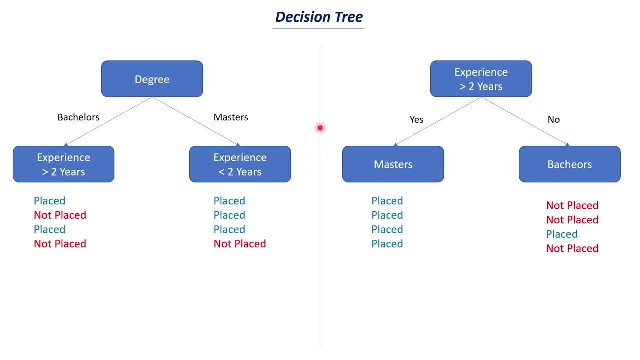 in this case, experience is my root node Right, So we need to determine which decision tree is best for making predictions And which is the best model when we compare these two. So this is where we use the measures such as entropy, information gain or Gini impurity. 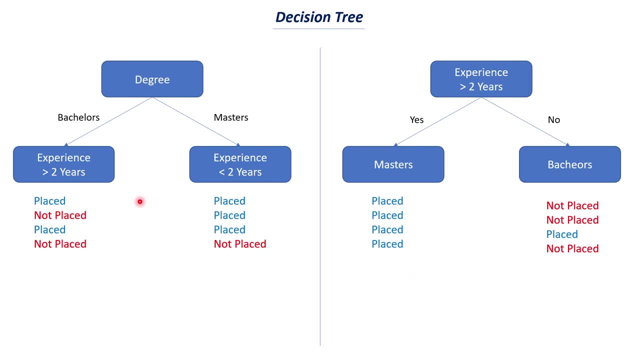 OK. So if you see the final output, you can see that in the first terminal node we can see that two people are placed and two people are not placed. So in this case three people are placed and one person is not placed. So in this second decision tree we can see that four people are placed. and you know, in 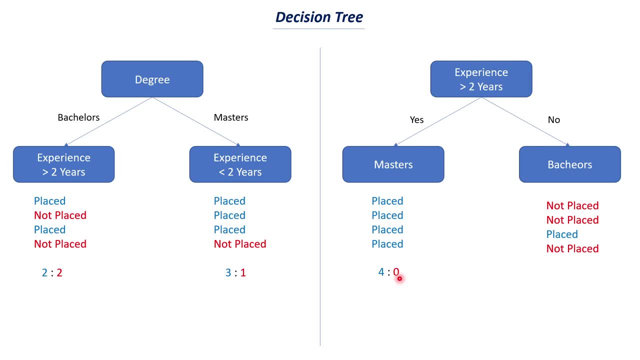 this case, four people are placed, So there is not anyone who is not placed in this case. and in this case, one person is placed and three person is not placed. So if you look at this, So in this particular case there is a mix of two classes. 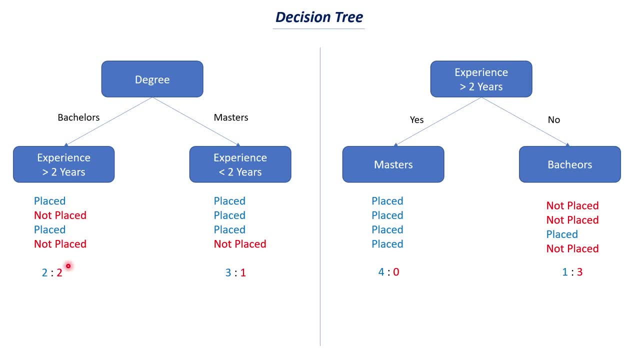 So, if you consider placed as one class and not placed as another class, So there is a mix of classes within this terminal node and in this case it is like three people are placed and one person is placed, and so on. So, if you see this, this is like a perfect segregation, because all the people in this 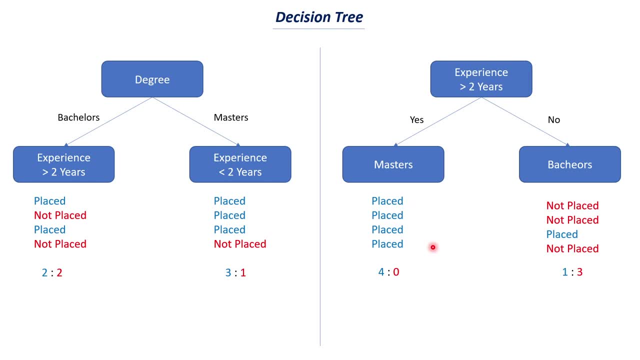 particular section are placed right. So we have to choose a decision tree that can split the classes into separate groups. So in this case it is separated completely, Right, Right, So we can call this decision tree, or we can say that this decision tree, where we have 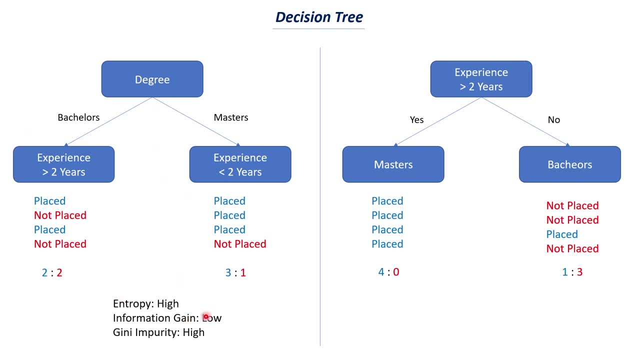 considered degree as root node, as I entropy, low information gain and I Gini impurity, whereas this decision tree will have low entropy value, I information gain value and low Gini impurity value. So we need to understand what is meant by these three terms. 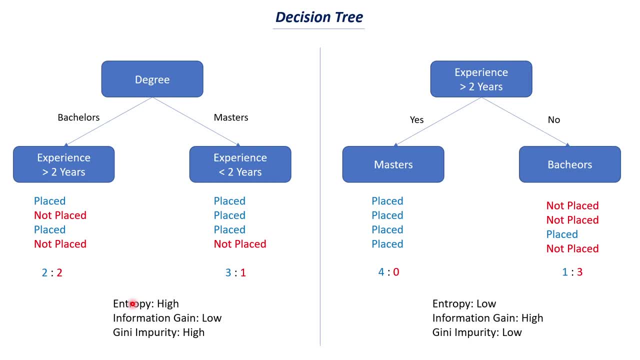 So entropy will basically tell you how random the data that you have. So in this case, if you can see, here there is not a clear split, So there is some randomness between the two classes that is present in the terminal node. So hence we can say that if the randomness is more, we can say that the entropy is high. 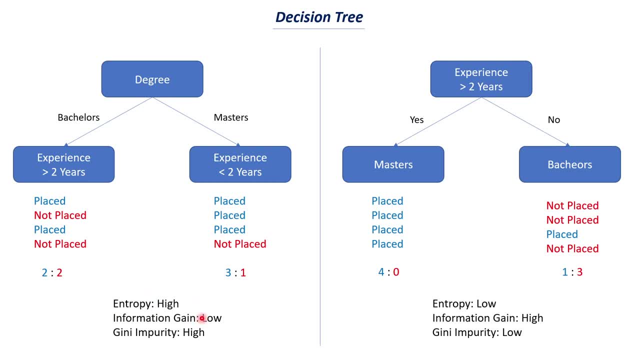 If the entropy is high, the information gain is low. So we will discuss in detail what is meant by this entropy and information gain and so on. But for now, understand that if we can split it, you know accurately, in that case the entropy will be low, information gain will be high, whereas the impurity will be low, whereas if 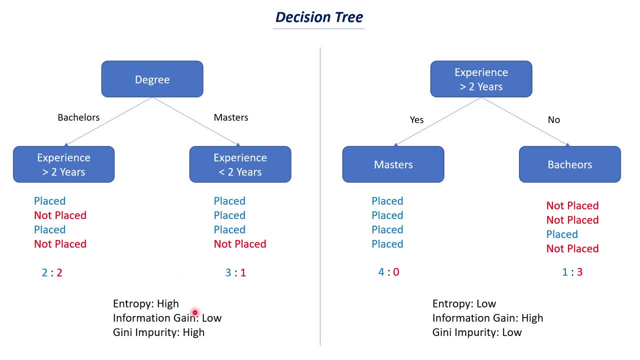 you cannot split it completely. the entropy will be high, information gain will be low. So these two, entropy and information gain, are almost like inversely proportional to each other. So let us try to understand. what does these three terms mean? So the first thing that we need to understand is entropy. 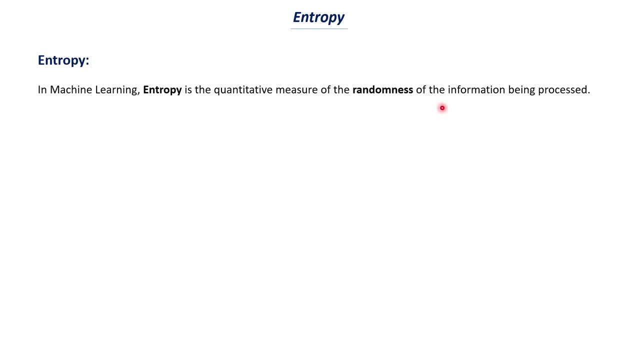 So in machine learning, entropy is the quantitative measure of the randomness of the information being processed. So entropy is a term that we would have studied in our school days in thermodynamics. So what we call entropy is that it is the disorderness of a system. 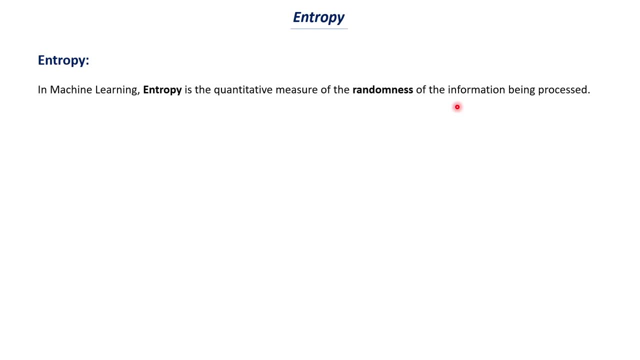 So in machine learning and mathematics, if we think about it, entropy is the randomness. So we are measuring this randomness in some quantitative measures. So we are measuring this randomness in some quantitative measures And it is the randomness of the information being processed. So if we consider this classification example that we have seen, 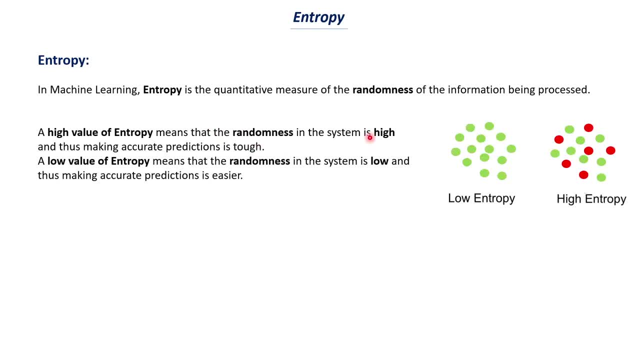 So we can say that I value of entropy means the randomness in the system SI. That means there will be mixing of the two categories, So there won't be, you know, separate segregation of the categories. So I value of entropy means the randomness in the system SI and thus making accurate 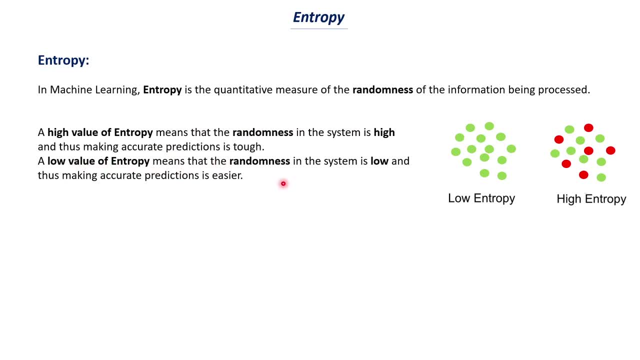 prediction is tough. A low value of entropy means the randomness in the system is low and thus making accurate predictions is easy. So if you see this image when you have low entropy, What we basically mean is, like that decision tree can separate the classes into two groups. 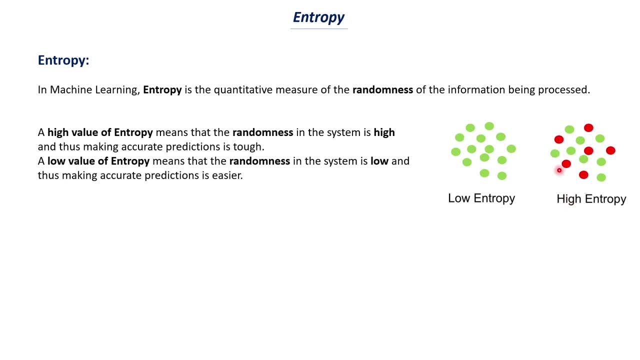 or something like that, Whereas if you have high entropy, that means the decision tree cannot build a decision system that can clearly separate the two categories. So this is what entropy means, And the formula for determining the entropy is this. So it is: the summation of I is equal to 1 and C. 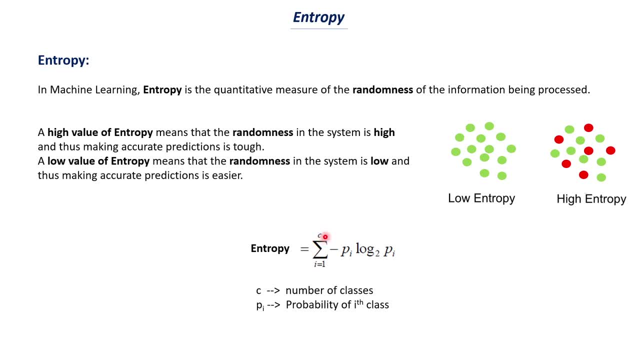 So C is basically the number of classes that you have. So in the example that we have seen we have two classes. Okay, So Let's say I is the probability of I class and log two of PA. So this is like the probability value. 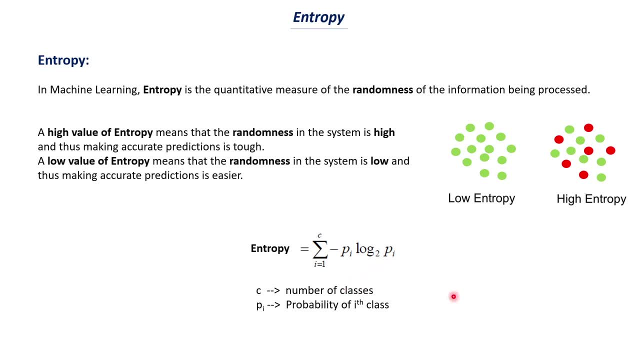 So probability is nothing. but so let's say that out of this, eight data points, So three people are placed and five people are not placed. So in that case, the probability of people who are placed is three by eight, Okay, Whereas if you consider the second class, the probability of people who are not placed is: 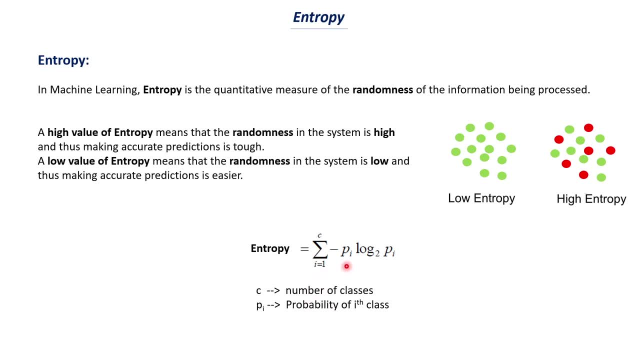 five by eight. Okay, So it is just the simple probability. So first we will take the probability of the class for placed people and we will find this particular value And we will add it with The probability of people who are not placed and we just need to submit. 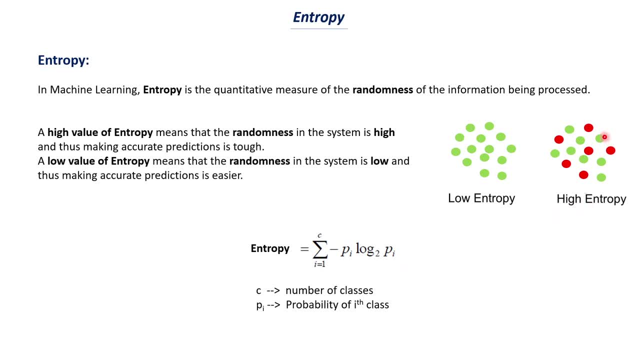 So this will be our entropy value, And if your entropy value is I, that means your decision tree is not working well because it can't classify the data points correctly. So if the entropy value is low, in that case it means it can clearly separate the values. 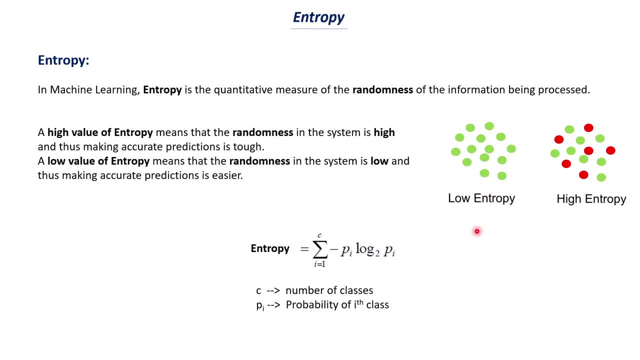 and it can you know, make good predictions. So our goal will be to choose the decision tree which has low entropy value And if we talk about, but you know, information gain. So the reason for finding this entropy is in order to determine how much information. 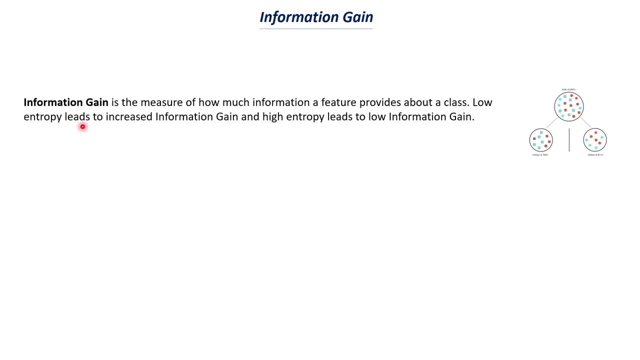 we can gain from the model. So, if we talk about information gain, information gain is the measure of how much information a feature provides about a class. Okay, So we are, as I have told you before, we are choosing different features for our root node and for our internal nodes for two cases of decision tree. 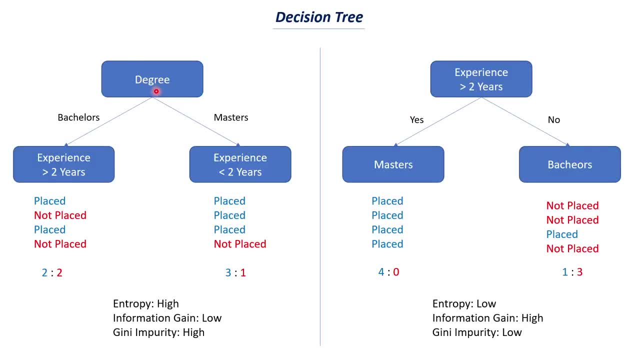 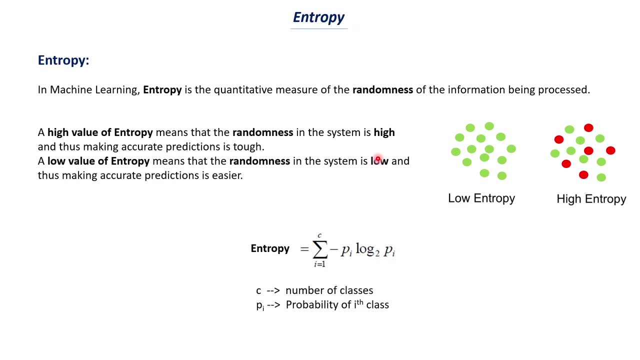 So if you just see in this case- So in the first example we have seen degree right as a root node and the second case, we have seen experience and the internal nodes has changed in both the cases right. So what we will try to do is, once we find this entropy, we need to find for which feature. 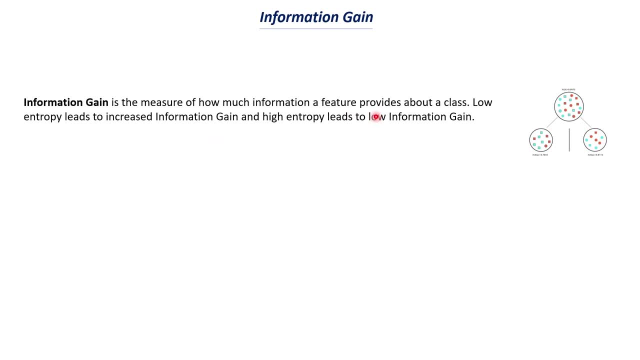 So if you for which feature you are selecting- a root node or the internal node- you are getting IE information again, IE information is the one where you are getting correct classification of data points. Okay, So information gain is the measure of how much information a feature provides about. 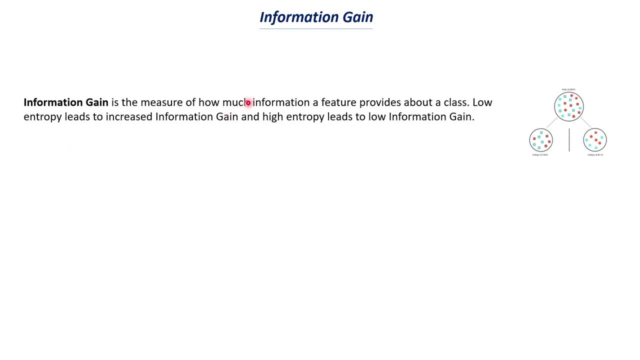 a class. Low entropy leads to increased information gain and IE entropy leads to low information gain, as I have told you. So if the entropy in the decision tree is more, that means it cannot give you a clear segregation between the classes. So the information you are getting out of it is kind of low. 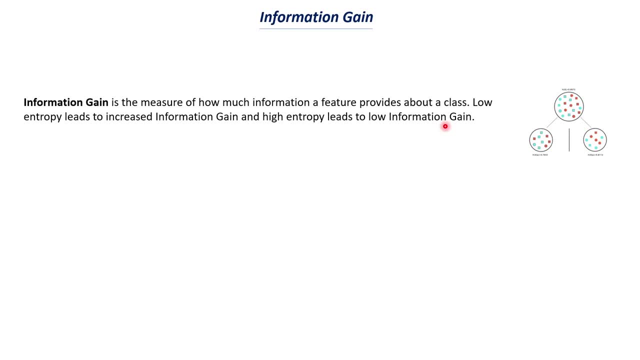 Whereas If you separate the classes separately, in that case it will have a low impurity and the information gain will be high. So information gain computes the difference between entropy before split and average entropy after split of the data set based on a given features. 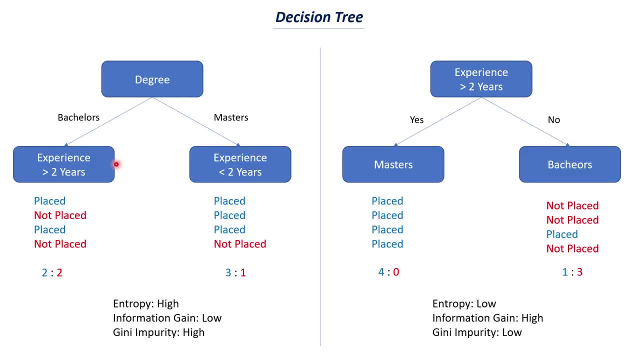 So how we will basically find the information gain is. so, before we split the data into these two categories or these two nodes, we will see what is the entropy at this particular stage once we split it based on the degree. So after that we will find again the entropy once the data has been splitted by the second. 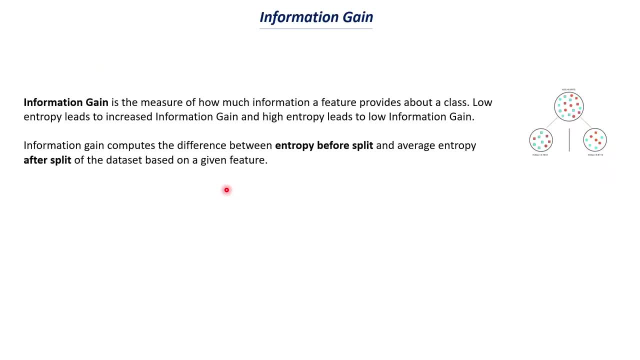 feature and so on. So first we need to see what is the entropy in the first case and what is the entropy in the second case, after the data has been splitted, and we just subtract it. So it is just finding the difference between the two entropy values. 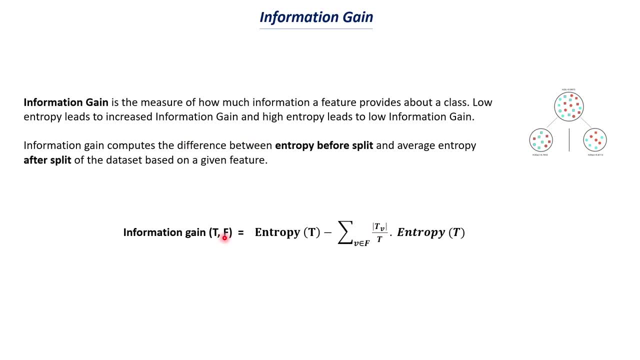 So this is the formula for entropy. So information gain of T, comma, F. So T is nothing but our target, the class that we are working on, and F tells the feature. So first we can take degree as the feature and we can find what is the information gain. 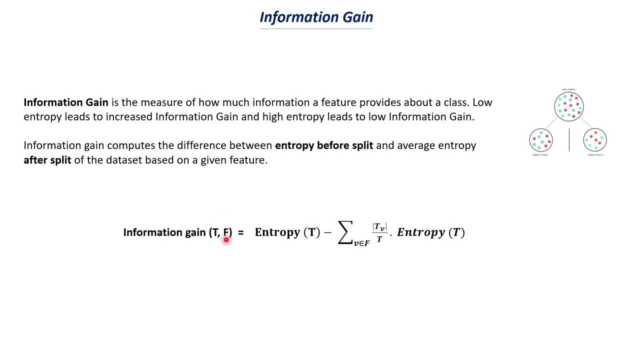 when we use degree as our root node And in the second case you can take the feature as experience in two years. So we will have two information gain and we will see which decision tree has the higher information gain value. So entropy of T is the initial entropy minus the summation of V of F. So it means like: 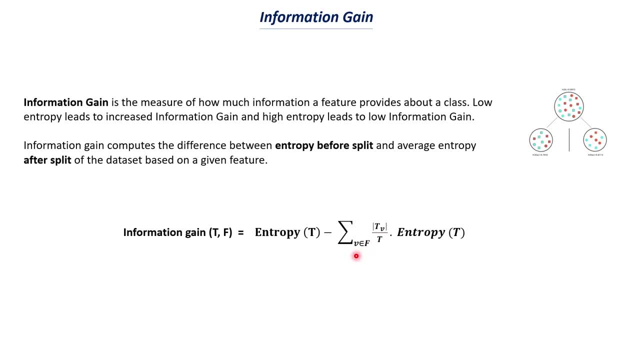 we have to take each values in that particular feature. So if you think about the experience in here, so we will take each of the values once we calculate the summation and so on. So T is T of V is nothing but the class or the target of that particular data point. 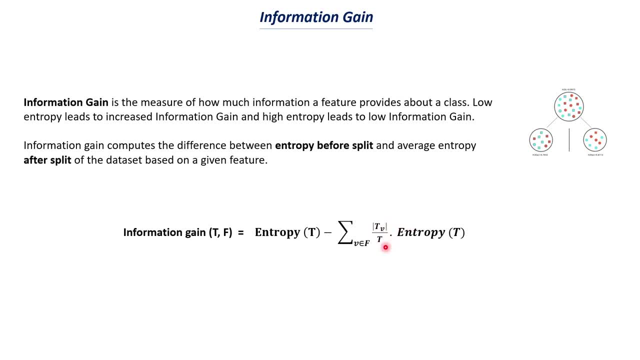 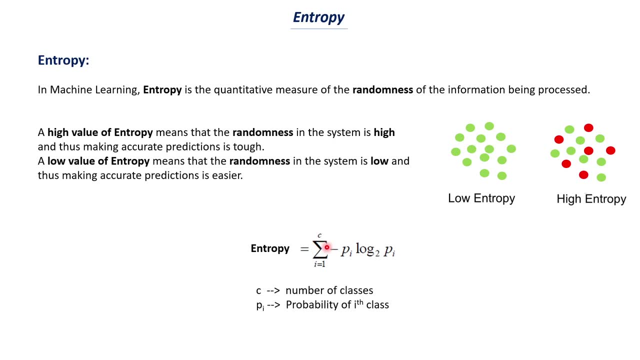 data point divided by the total number of class that you have. so it is just similar to the probability that we have seen before, and then we have to multiply it with the entropy of t, and we have seen the formula for entropy of t here, right, so i'm not going to go in. 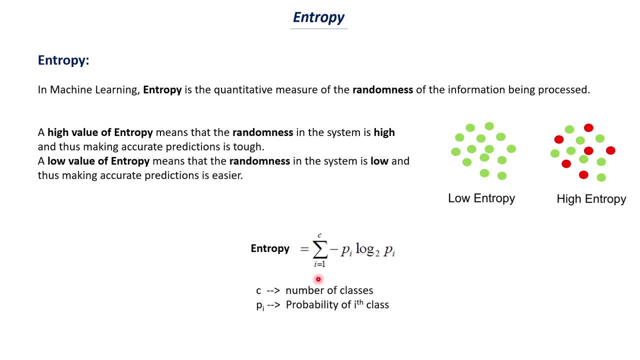 detail about how we get this entropy formula and so on. so that is like out of scope for this particular video, but you can find several examples on the internet where you can have some sample data set and you can manually calculate the entropy values and information gain value. so you can do that in order to understand how to calculate this values. what 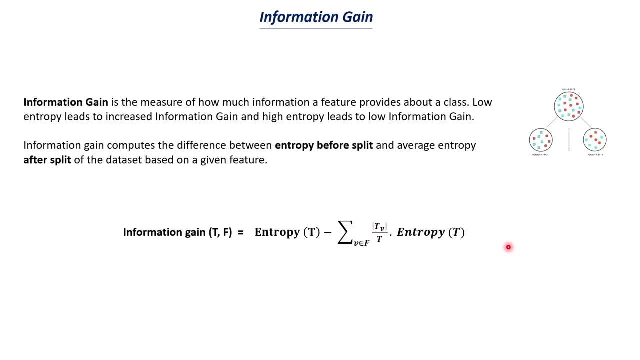 is the range and so on. okay, so entropy is about uh, calculating or measuring that randomness in the data set or the decisions made by the decision tree. and information gain is what is the amount of information we are getting for a specific feature, that we are choosing our root node and 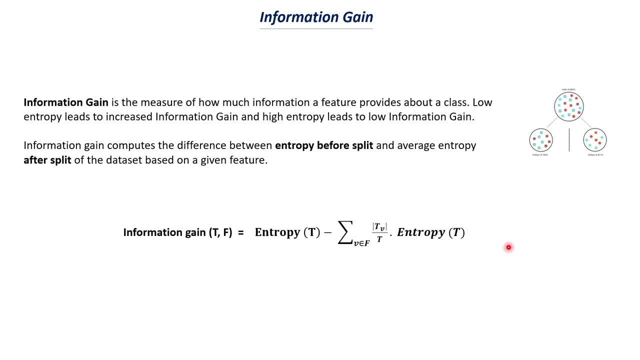 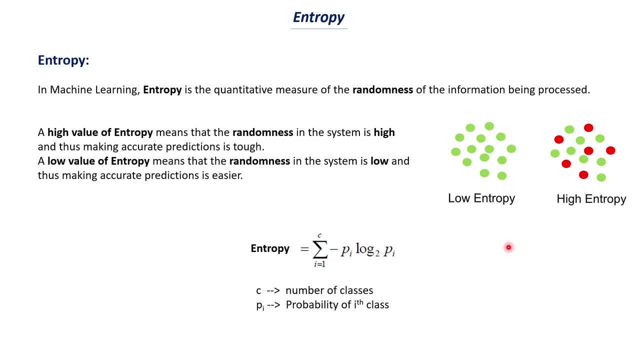 internal node. so this is about information gain. and finally, we are genie impurity, so we you can think about entropy and information gain together. so we determined entropy in order to find our information gain, and genie impurity is a separate concept. okay, so the split made in a decision tree is said: 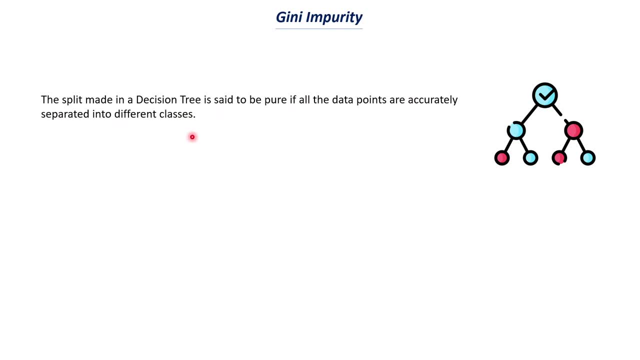 to be pure if all the data points are accurately separated into different classes. so, as we have seen in the previous example, let's say that we are building a decision tree and it can clearly separate the people who are placed and people who are not placed, using different nodes and 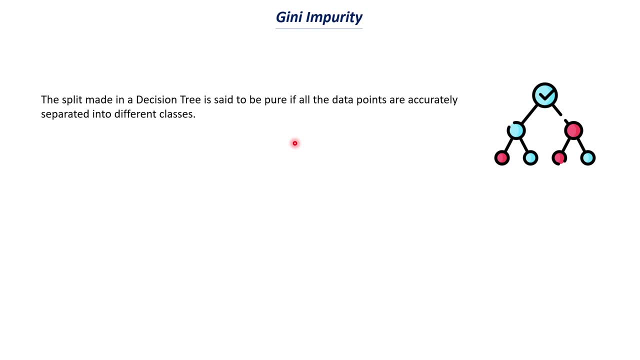 internodes. so in that case we call the decision tree as pure, because it doesn't have any inter mixing of classes. if it has some inter mixing of classes, if it contains, you know, in the terminal node there are people who are placed and not placed in the 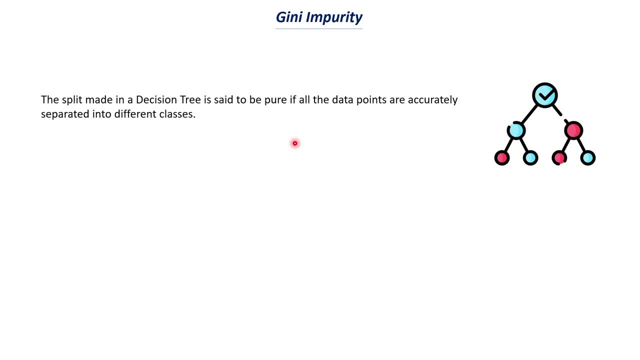 terminal node. so in that case the decision tree is said to be having some impurity and the measure of this impurity is called as genie impurity. so genie impurity measures the likelihood that randomly selected data point would be incorrectly classified by a specific node. let's say that we. 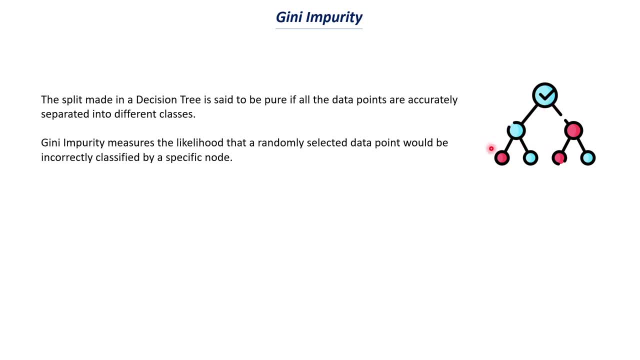 have built this nodes here, root nodes and internal nodes and so on. so if you choose a random data point and you are plugging in the values in this particular decision tree and we are finding what is the likelihood that it is going to be deterred or it is going to be predicted? 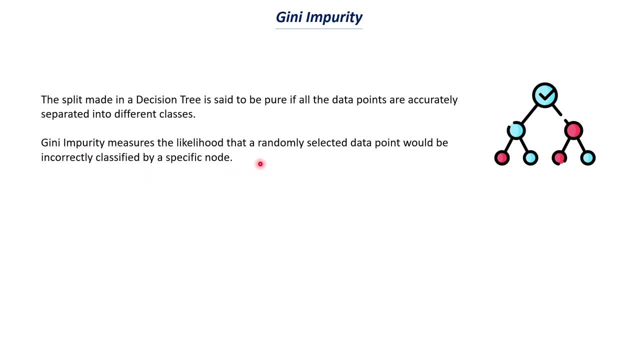 wrong class. okay, so that is the measure of this genie impurity. so this is similar to the last function that we have worked on, but this is like more uh involved in the uh categorical data. so you just take a new data point and we are going to find what is the probability that it is going to. 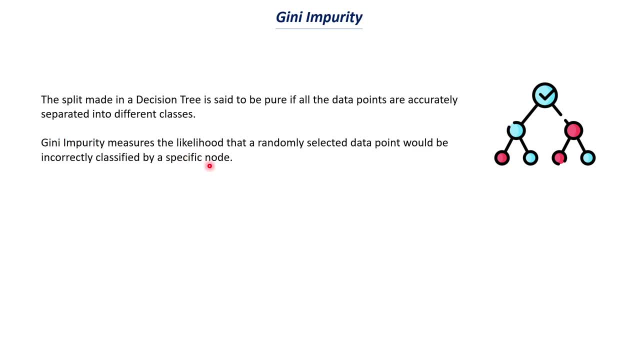 be predicted wrongly, because this is impurity, okay, so we need to find what is the chance we are going to get a wrong classification. so that is, uh, the measure of this genie impurity, and this is the formula for genie impurity. so it's g is equal to summation of i is equal to one c, so c is nothing. 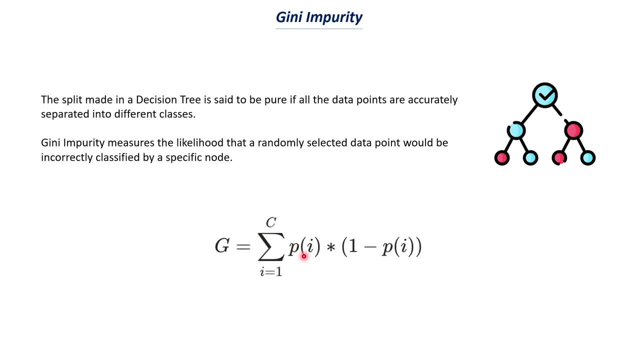 of classes that we have, and p of i is again the probability of that particular class. so if there are 15 people and out of those 15 people let's say that seven people are placed, so for class placed the probability will be 7 by 15, or, you know, 5 by 15. so based on the number of data points we have, 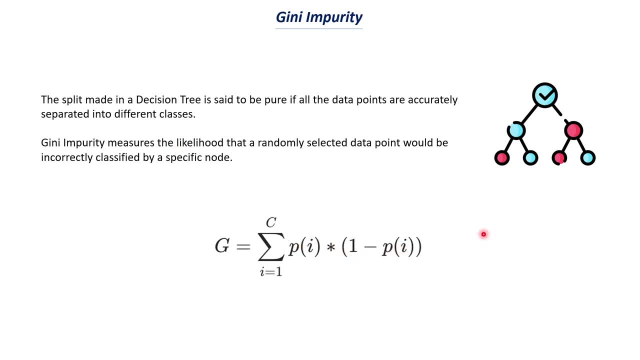 so into 1 minus again p of a. so this is the formula for genie impurity. so if you think about entropy, uh, it is like: uh, what is the randomness? so how much? uh, the classes are mixed with each other, so that is called as the entropy and based on this entropy we find the information gain. 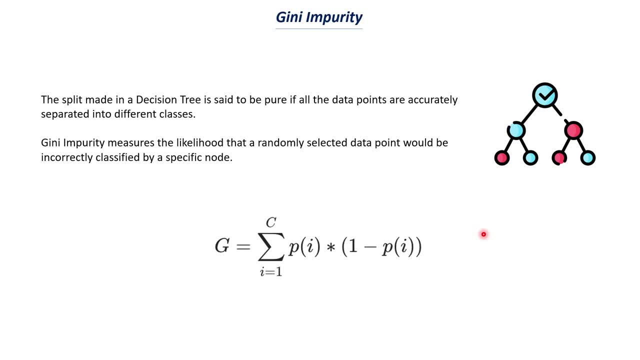 whereas the genie impurity is the likelihood of- uh, you know your model predicting a class wrongly, so you have to understand this clearly, okay, so these are all the three things that are very important when we are building our decision tree, because, like, if you use a decision tree in sk, learn. 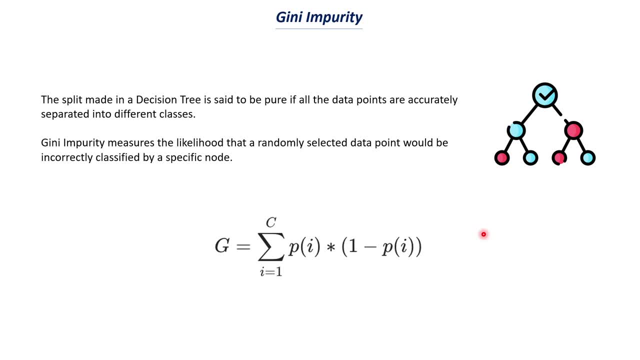 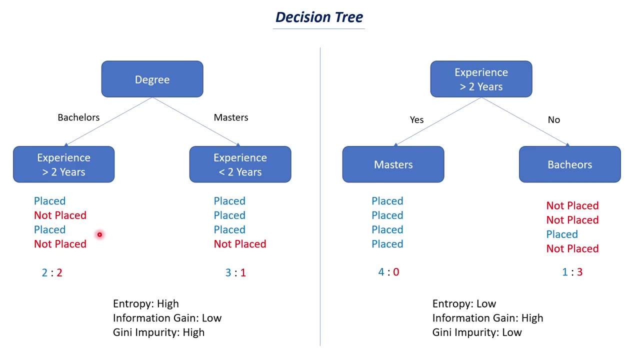 there is an uh parameter called as criterion, where we have to specify whether we want to build a decision tree based on the entropy measure or with the genie impurity measure. okay, so we can choose either between this information gain or genie impurity. okay, so now, if you see this, we can see that in this case, uh, there is some mix of classes, right? so we 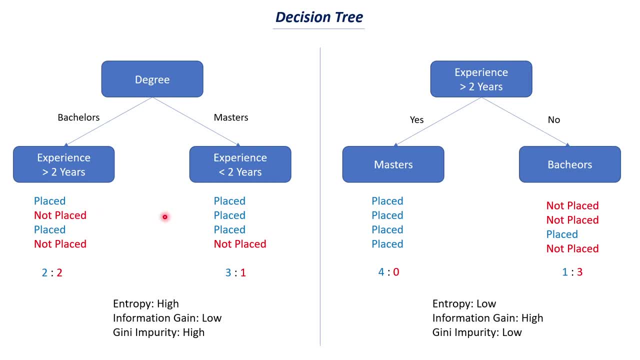 have people who are placed and not play, so there is not a clear segregation between them. so we can say that this decision tree is not that much pure, so there is some impurity. so this will have a i genie impurity value and because there is some randomness in the placed and not placed people. 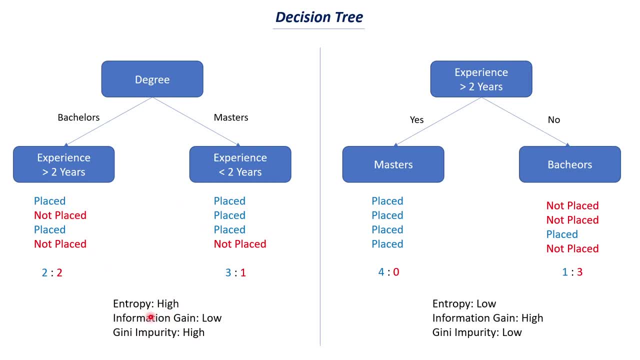 we say that there is an i in entropy. so whenever there is an i entropy, the information gain value will be low and in this case- you can see here there is some intermixing, but the intermixing will be low compared to this decision tree. okay, so in this case we can clearly segregate all the 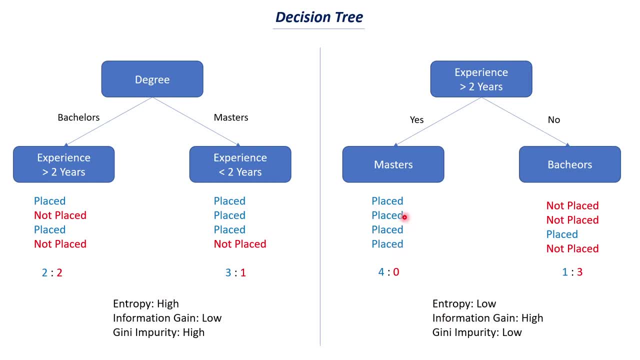 people who are placed. okay, so in this case the purity will be i, because we don't have any intermixing. so the genie impurity value will be low and your entropy value will also be low, because the randomness is quite uh decreased. so in this case we have one placed person, uh, among uh three.